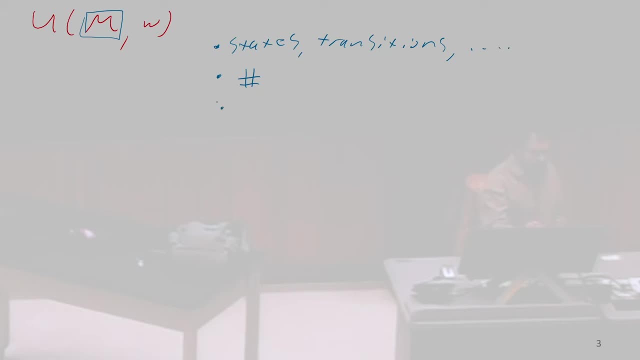 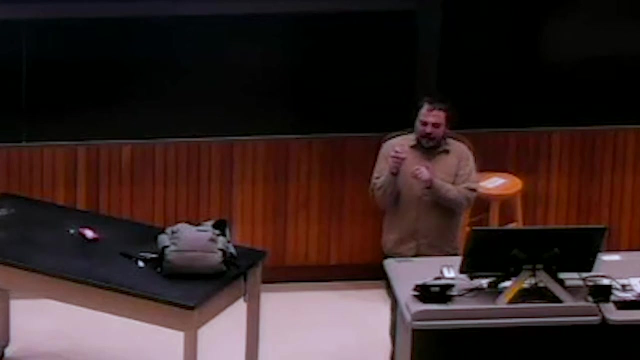 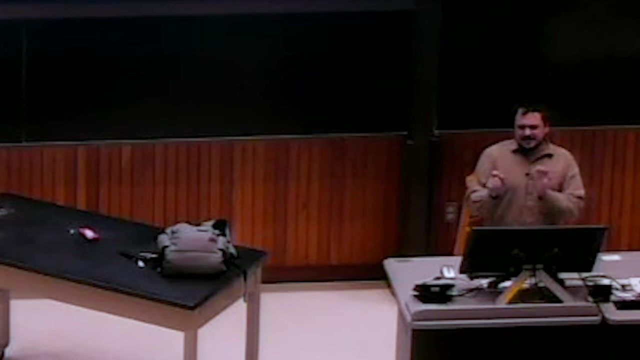 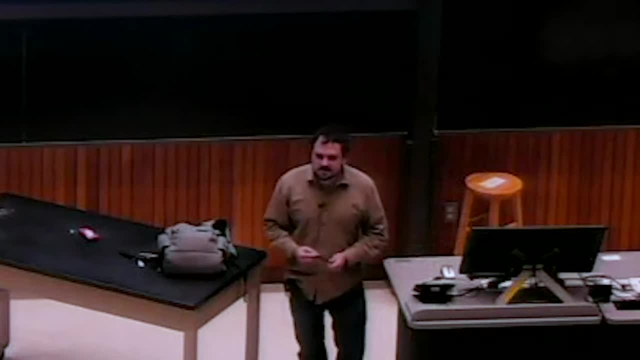 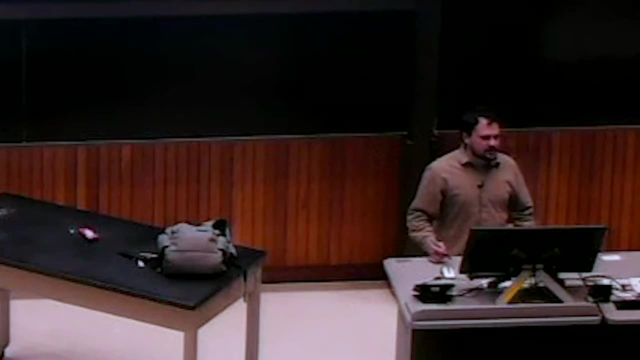 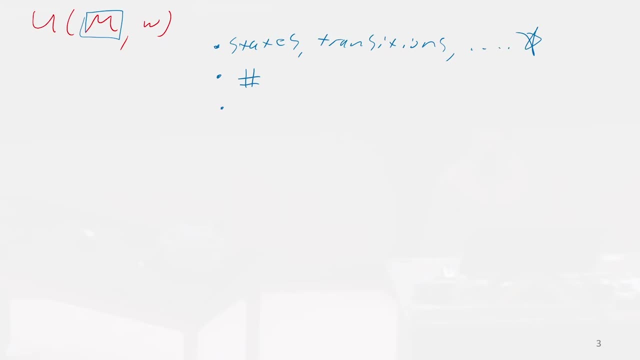 Something that we are going to prove. we're going to sort of take this for granted today. we're going to prove it either Wednesday or next week, depending on how fast we go. is that also things like Python? We could have this idea of like an idealized Python that we could think of as describing 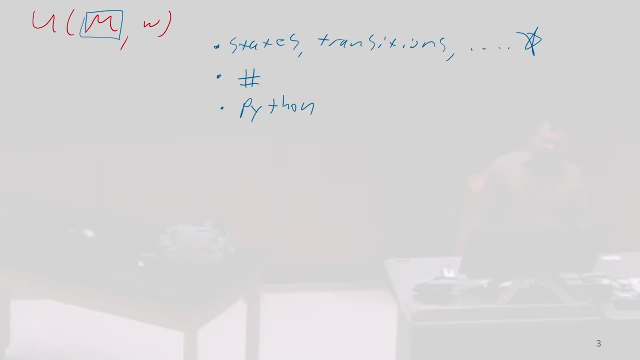 a Turing machine. So when I say idealized Python, we have this issue with Python where, like, you've actually got a fixed word size on your computer that limits how much memory you could possibly have. So idealized Python is kind of how you think about Python when you're programming it as 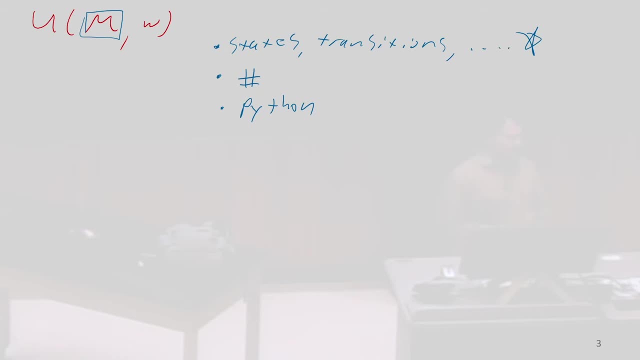 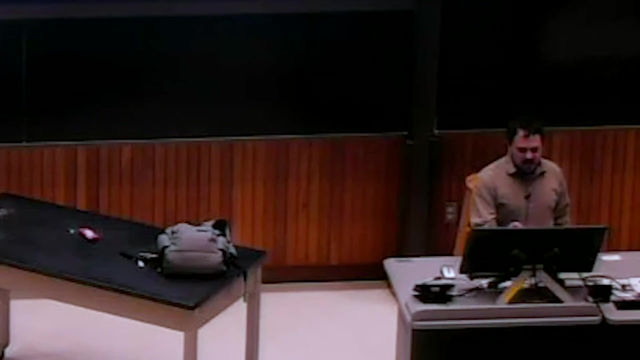 if numbers have infinite precision and lists can be unlimited size and so forth. So the way you typically think about Python- you don't worry about memory constraints and so forth- That version of Python that you have in your mind, you can think of that as a description. 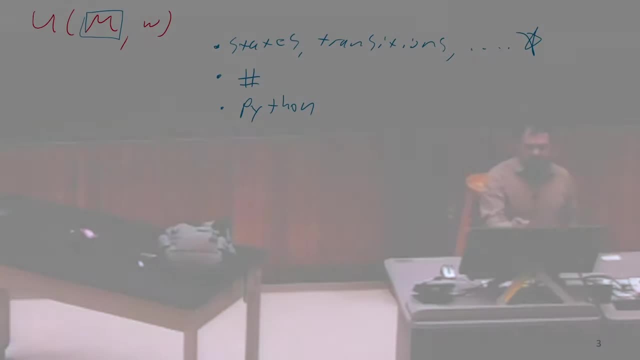 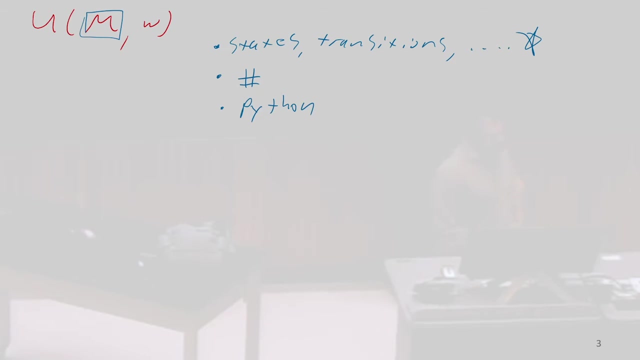 of a Turing machine. It's a more sophisticated description than states, transitions et cetera, But it is still just describing a Turing machine. So everything that we're going to talk about today that works for states, transitions et cetera, as being a description of our Turing machine, it's going to equally apply and in 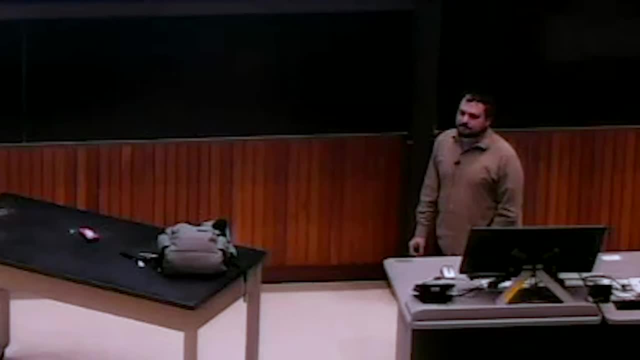 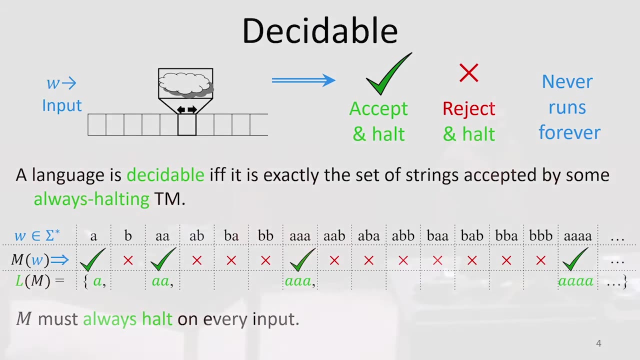 a very similar fashion with Python code. With Turing machines, there were three options for what a Turing machine could do for a particular input. It could have been that that Turing machine halted, And when it halted it was a Turing machine. It was going to either accept that input, that is, return one for that input- or reject. 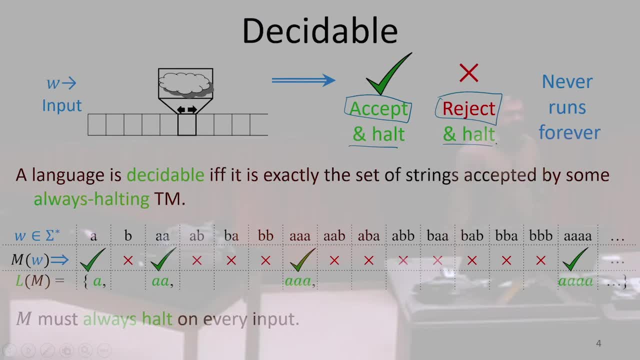 that input. so still halt and reject. so that is return zero for that input. Or there was sort of this third option where it never returns, that is, it runs forever. There are three behaviors that a Turing machine can have for one input. 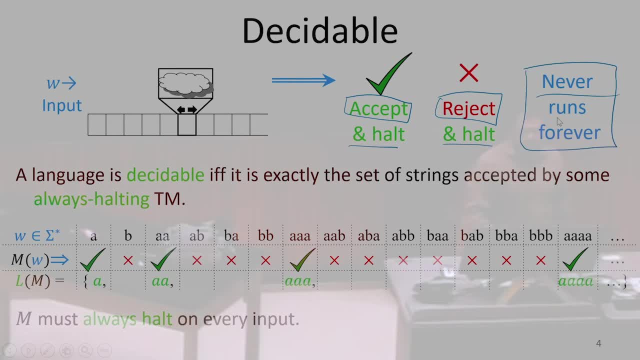 It halts and then accepts, it halts and then rejects, and then it runs forever, And what I'm going to do is I'm going to give you a couple of definitions of some things that might come in handy. So we're going to say that a function or a language is decidable. 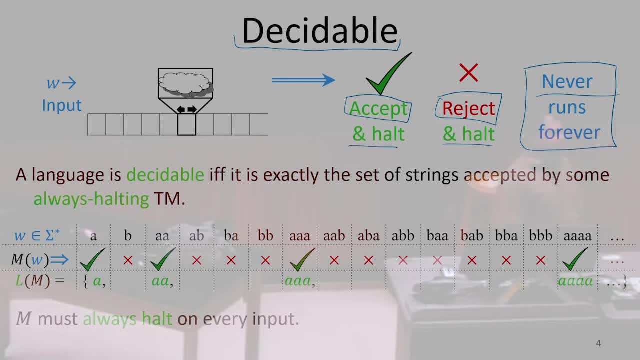 So we mentioned last time we could consider a language to be the set of all inputs for which that Turing machine returns one or accepts. So we can say a language or a function is decidable, provided it can be computed by some always halting Turing machine. 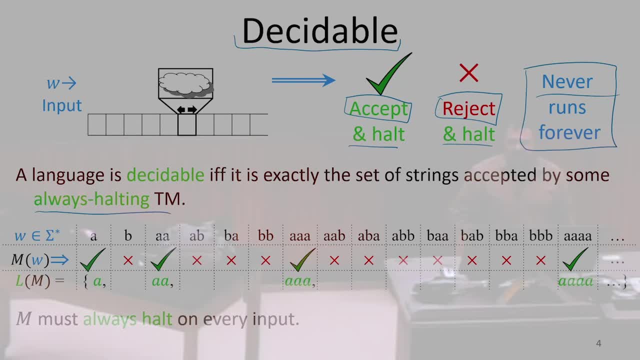 If I had some language and I want to know: is it decidable? What I would do is Ask this question of: is there some always halting Turing machine that accepts exactly all of the strings in that language or returns one for exactly the right things? 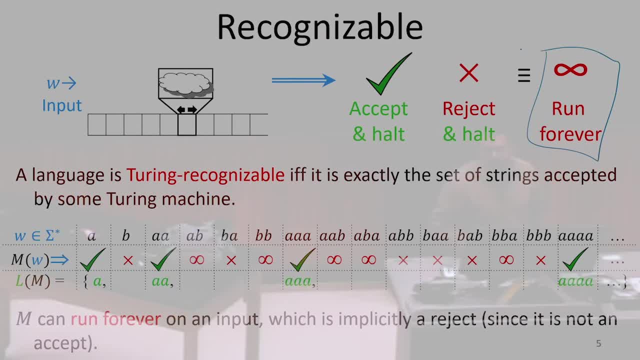 Alternatively, if we have this run forever answer, if we allow for this, then we're computing things that we call recognizable. recognizable things are ones where all of the things that we ought to return one for, or all of the things that ought to be in our language, we can. 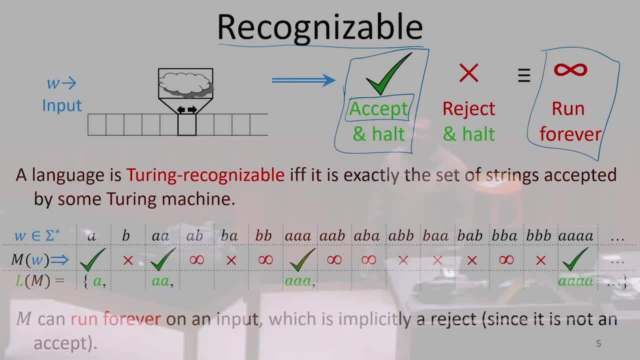 find a Turing machine which is going to accept and halt for all of those, for all of the things that we want to return, one for all of the things that belong to our language. we're going to halt and accept for all of those but things that aren't in the language we can either halt and reject or run forever.